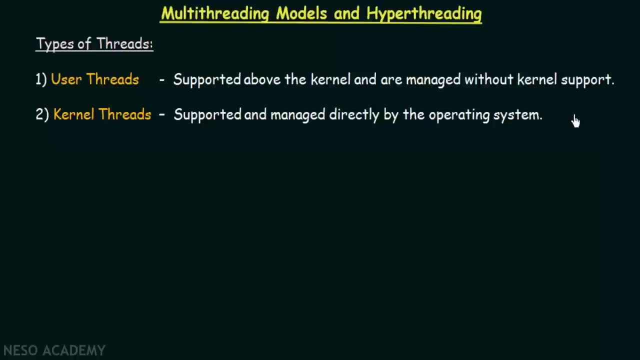 So kernel threads are the threads which are managed directly by the operating system and not by the user. So these are the two types of threads that we have. So when we started studying, when we started studying about operating system, we saw that the users are constantly interacting with the system. 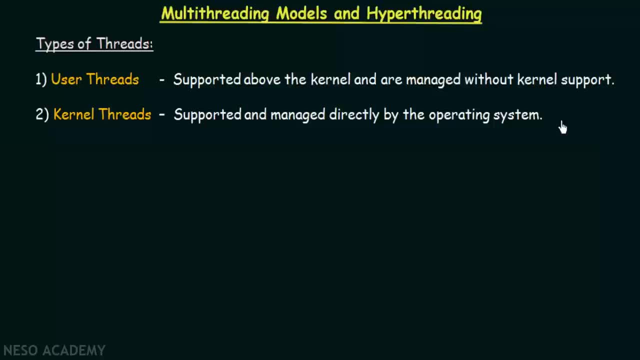 And the operating system is what allows this to happen. So, since we have seen that there are two types of threads- the user threads and kernel threads- So for these two threads to be able to function together, there must exist a relationship between the user thread and kernel threads. 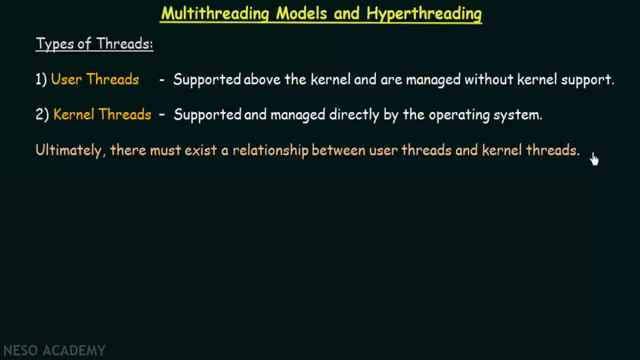 So, ultimately, for the system to function, there must exist a relationship between the user threads and the kernel threads. So we will see how we can establish this relationship between the user threads and the kernel threads. So that is the thing that we are going to study in multi-threading models. 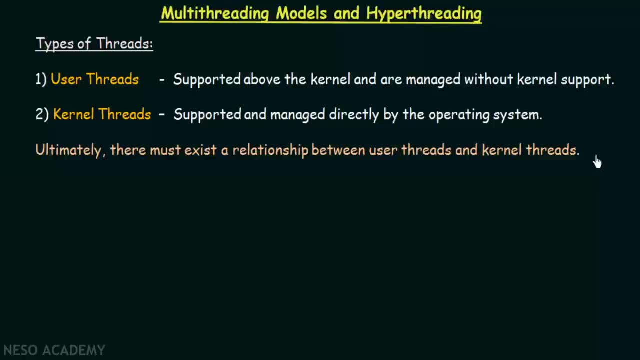 So multi-threading models are nothing but the type of relationships that can be there between the user threads and kernel threads. So we will see what they are. So there are three common ways of establishing this relationship, And what is this relationship? 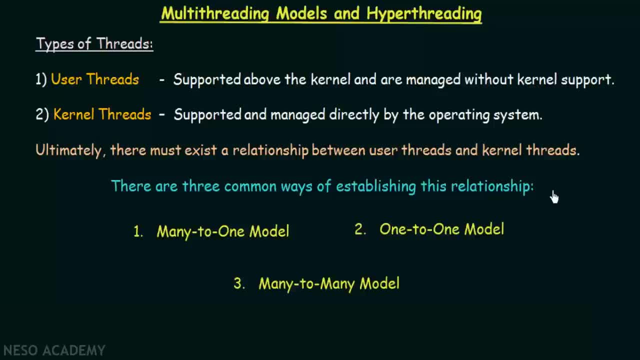 The relationship between the user thread and the kernel threads. So let's see what they are. The first one is many-to-one model, The second one is one-to-one model And the third one is many-to-many model. So we will see each of these models one by one. 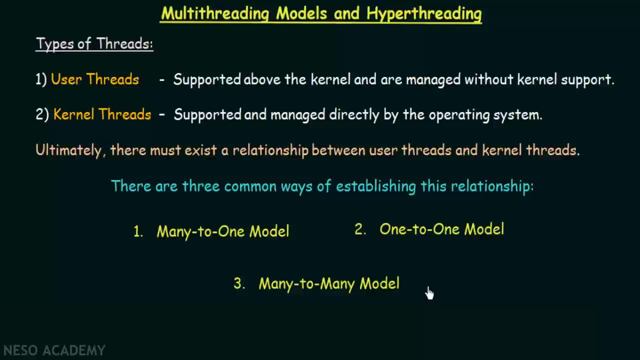 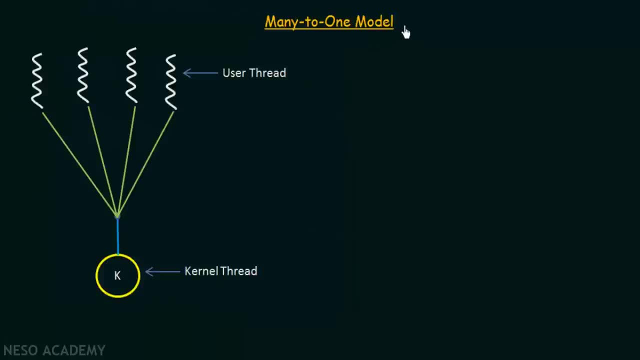 And we will see how do they function, what are their limitations and which one among these are the best. So, coming to the first model, we have the many-to-one model. So from the name itself we can understand that there is a many-to-one relationship. 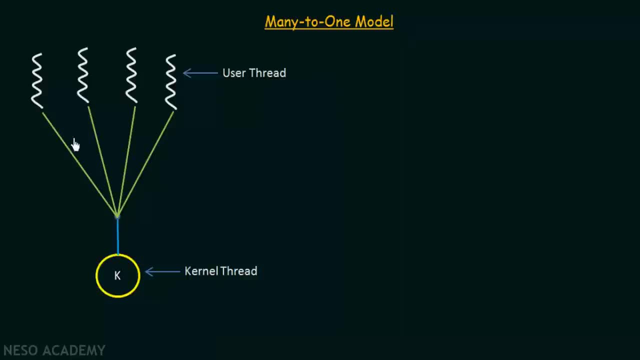 established between the user threads and the kernel threads. So from this diagram we can see these things: on top they represent the user threads And then the circle over here it represents the kernel thread. So we see that many user threads are associated to one kernel thread. 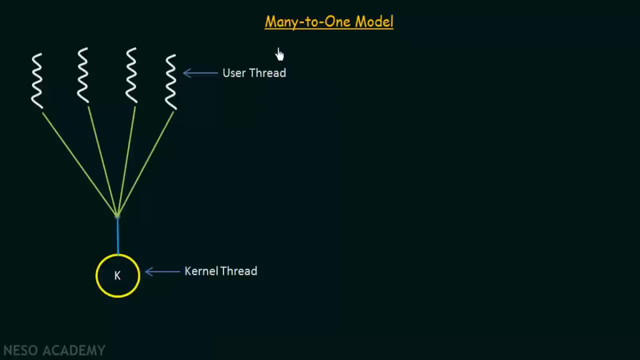 Or many user threads are accessing one kernel thread. So that is what we mean by the many-to-one model: Many user threads to one kernel thread. So, as I told you, in this model it maps many user level threads to one kernel thread. 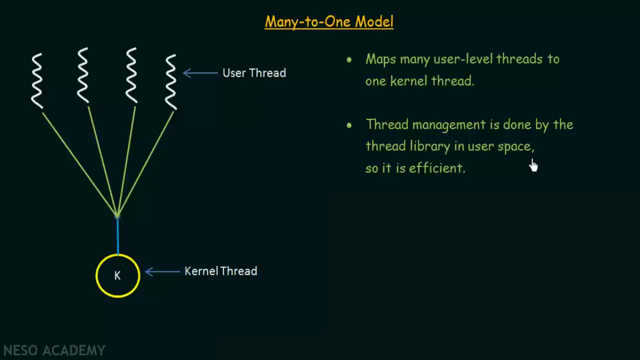 And then the thread management is done by the thread library in user space. So it is efficient. Thread management is done in the user level, not in the kernel level. So in that way this is efficient because we are able to manage the threads in the user space. 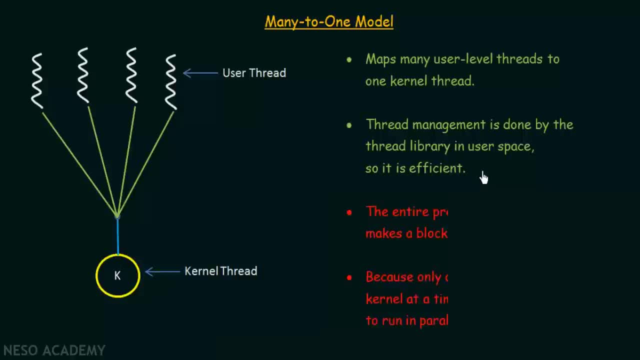 Now let us see what are the disadvantages or the limitations of this model. So here are the limitations: The entire process will block if a thread makes a blocking system call. So we see that many user threads are associated or mapped to one kernel thread. 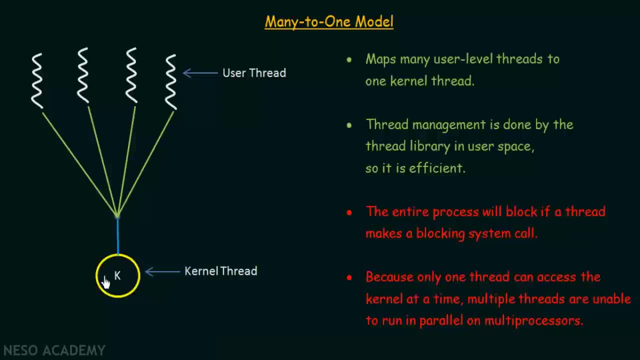 If one of the threads makes a blocking system call, then the entire process will be blocked, Because let's say that all these threads are associated to one single process. They are the threads of one single process doing a certain task And all these threads are mapped to this kernel thread. 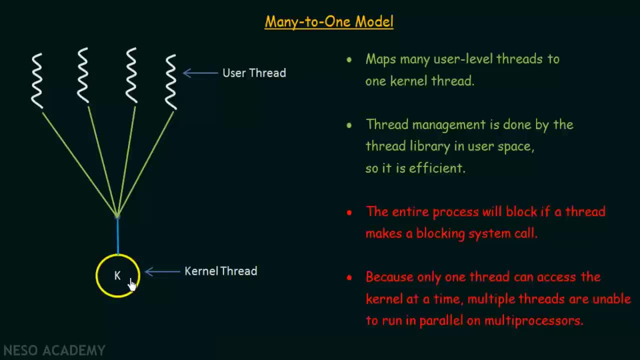 in the operating system. So let's say that one of the threads makes a blocking system call. So if that thread makes a blocking system call, this kernel thread will be blocked, And if this is blocked, then all of them will be blocked. 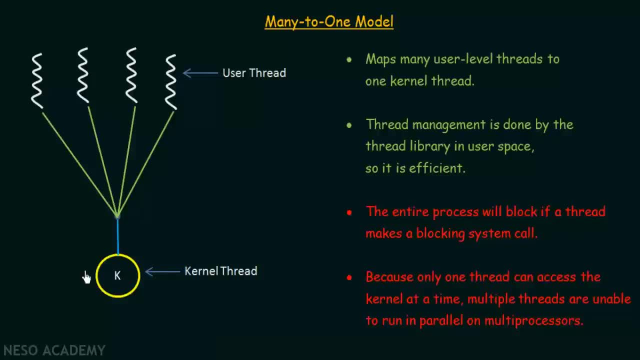 because they are not connected. They are all mapped to this single kernel thread. So that is one of the limitations or disadvantage of this model. So if one thread makes a blocking system call, the entire process will be blocked. And then the second limitation is that 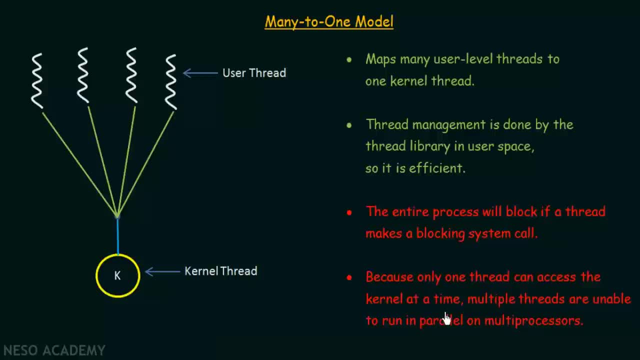 because only one thread can access the kernel at a time. multiple threads are unable to run in parallel on a multiprocessor. So, as you see here, since these multiple threads in the user level are mapped to just one kernel thread, even if we are having a multiple 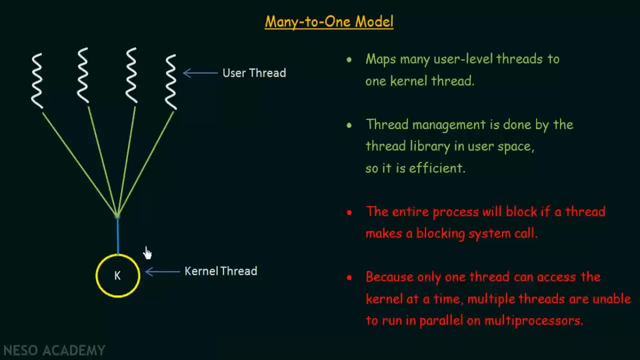 system. if you are having a multiprocessor, we are not going to be able to make use of that multiprocessor system, Because even though we have multiprocessor, that means even though we are having more than one processor- one kernel thread will. 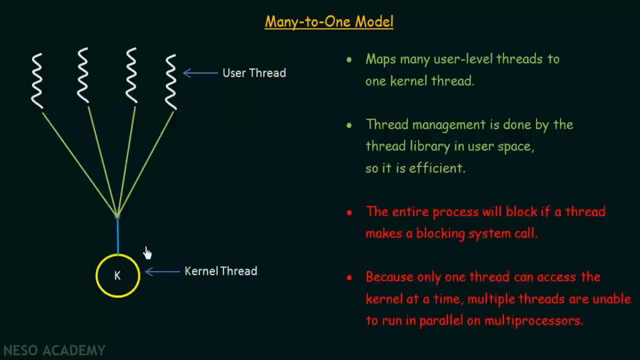 run only in one of the processors. One kernel thread cannot run in two processors. So even though we have many processors, this entire thing will run only in one of the processors because they are all mapped to one kernel thread and one kernel thread will run. 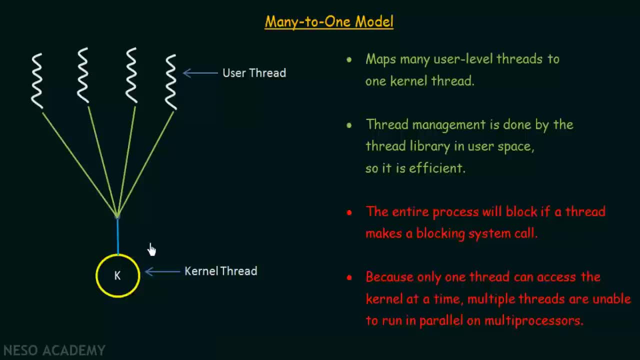 only on one of the processors. So that is another limitation of the many-to-one model. Alright, so now let's go to the next model and see how is that better than this, and if that has any limitations as well. So the second model that we have is: 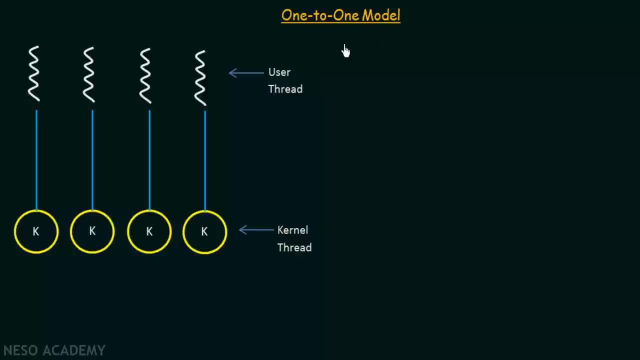 one-to-one model. So from the name itself even here we can understand here that one user thread is mapped to exactly one kernel thread, Unlike the many-to-one model. here one user thread is mapped to only one kernel thread. So here this user thread is mapped to. 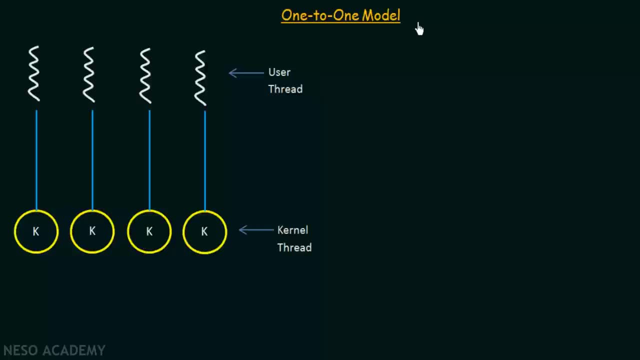 this kernel thread, this one to this one. So let us see how does this work and what are its benefits and what are its limitations. So, as I told you, in this model it maps each user thread to one kernel thread and then 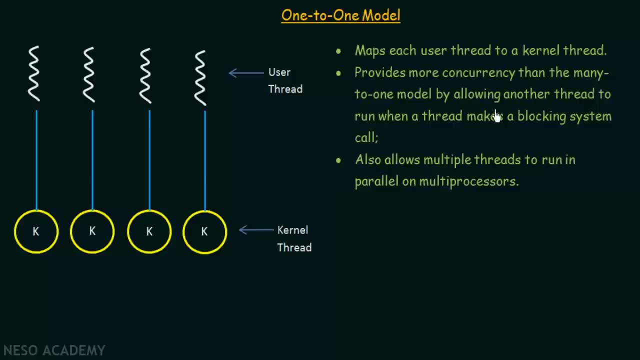 it provides more concurrency than the many-to-one model by allowing another thread to run when a thread makes a blocking system call. So in this case, even if one user thread makes a blocking system call, the entire process will not be affected, unlike the many-to-one model. 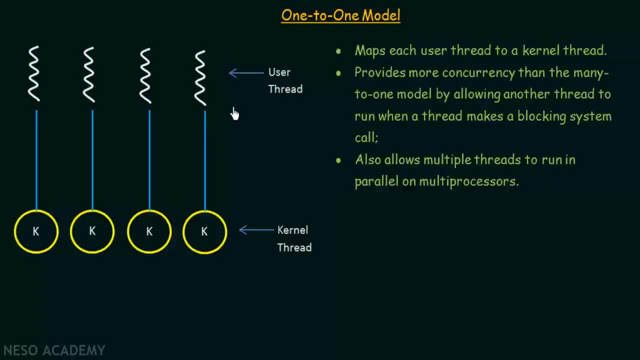 So here let's say, for example, that these four threads belongs to one process, and then let's say that one of the user thread makes a blocking system call. So if it does so, only this kernel thread associated with this user thread will be affected. 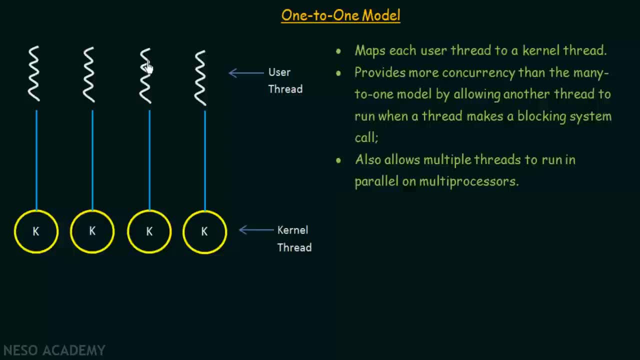 and only this part will be blocked. So the other part of the process, that means these three threads associated with these three kernel threads, can still run, even though this had made a blocking system call. So that is one advantage as compared to the many-to-one model. 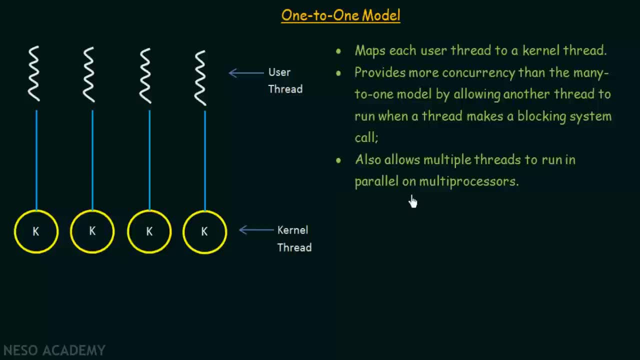 And also it allows multiple threads to run in parallel on a multi-processor. So in the previous one we saw that we cannot make use of the multi-processor system, But in this case we are able to make use of multi-processor system. 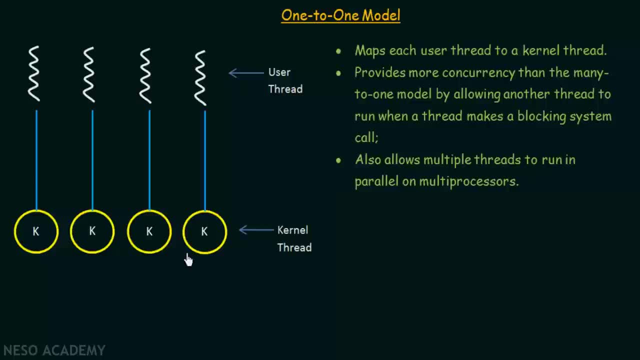 Why? Because each user thread is associated to one kernel thread, So each of these part can run on one of the processors that we have. So suppose we are having four processors in our system. then each of these threads can run on one of the four. 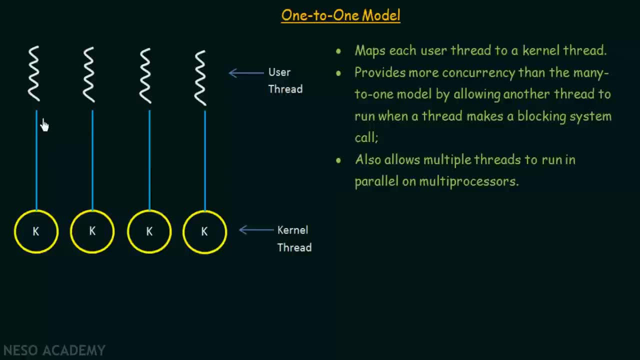 processors, So this one can run on one, this on another one, and so on. So we are able to make use of the multi-processor architecture that we have in case of the one-to-one model. So so far we saw that. 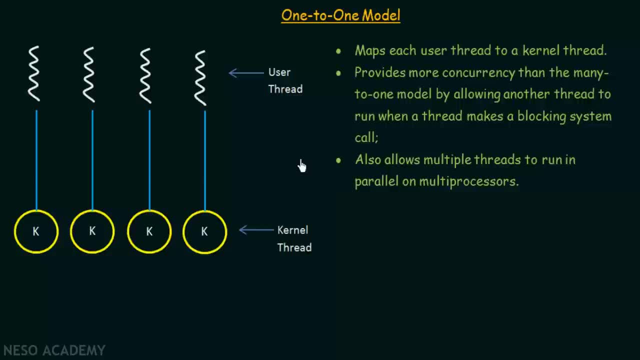 one-to-one model is having some advantages as compared to the many-to-one model. Now let's see if it has some disadvantages. and if they have, what are they? So here are the disadvantages: Creating a user thread requires creating the corresponding kernel thread. So here we. 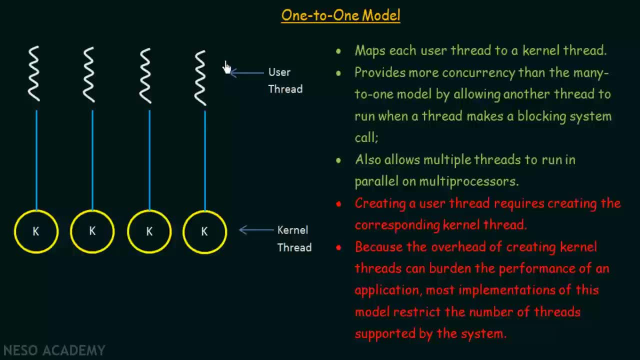 see that each user thread is mapped to one kernel thread. So whenever you are creating a user thread you have to create the kernel thread as well. So that may become costly sometimes And because the overhead of creating kernel threads can burden the performance. 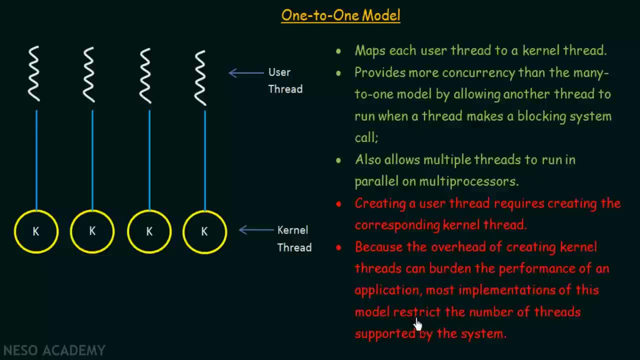 of an application. most implementations of this model restrict the number of threads supported by the system, So the overhead of creating kernel threads can sometimes be very heavy on the system or the application that is running. So what happens is that most of the applications they will restrict. 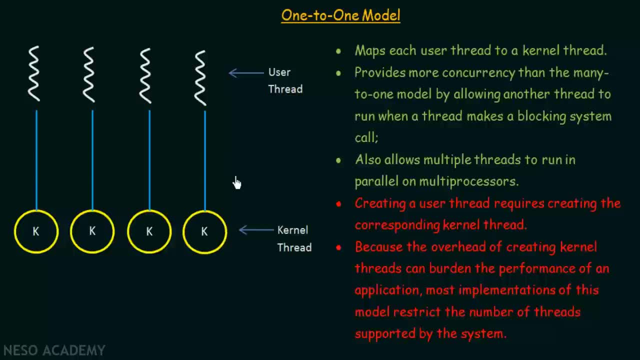 the number of kernel threads that can be created, Because in one system there is a limit of how many threads can run at a time. So if you are having a multi-processor system with four processors, then at a time only four threads can run, because 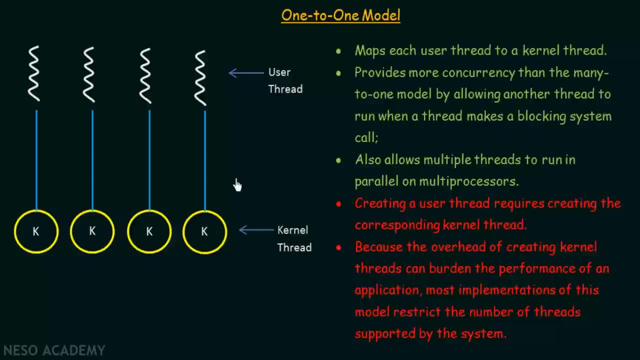 each thread will run on one of the processors. So if you are having a processor with four cores, that means if you are having four processors in your system, and if you are having five threads and trying to make those five threads run at the same time, it may not work. So the application. 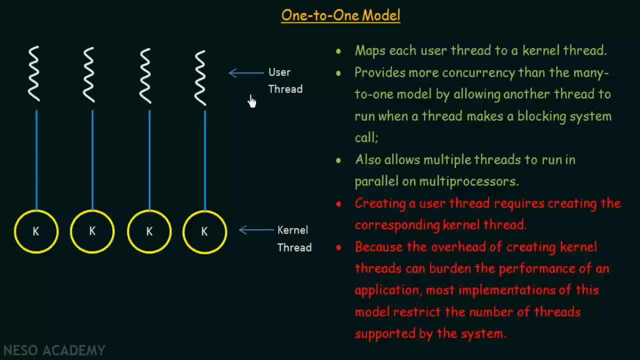 may have to restrict the number of threads that are supported, So that is another disadvantage of this one-to-one model. Now let us go to the next model and see if that is better than these two that we have discussed till now. So here we come to the last model. 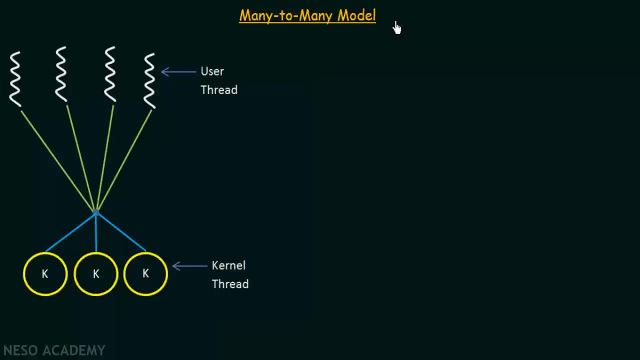 which is the many-to-many model. So here again, from the name we can understand that many user threads are associated or mapped to many kernel threads. So from the diagram it is very clear: Here we have the user threads and here we have 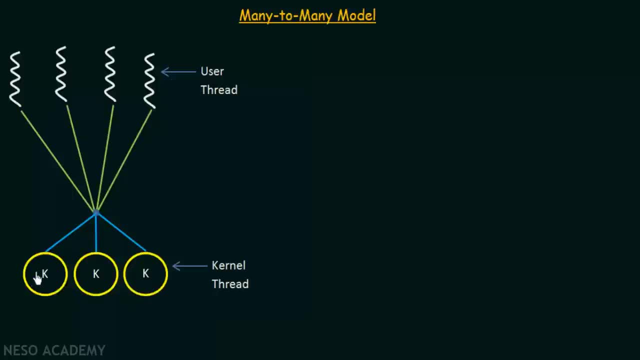 the kernel threads And these user threads are associated with these kernel threads or they are mapped to these kernel threads, So there is a many-to-many relationship in this model. So let us see what are the advantages of this model and if this 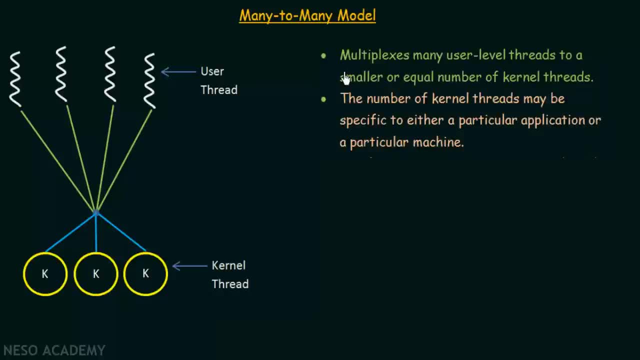 is better than the other two that we have discussed. So here, as I told you, in this model it multiplexes many user level threads to a smaller or equal number of kernel threads. So, as we see, here there is a mapping between many 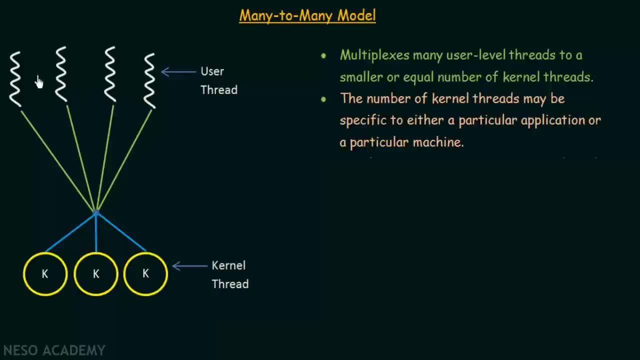 user level threads to a smaller or equal number of kernel threads. So here we have four user threads, and they may be mapped to four or lesser number of kernel threads. That is what we mean by this. And then the number of kernel threads may be specific to either a 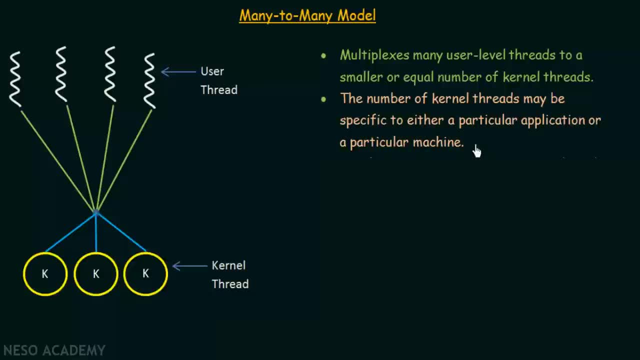 particular application or a particular machine. So, as I told you, there is limitation of the number of threads that we can have in a system. So the number of kernel threads that we can have in this model, it may be specific to a particular application or a particular. 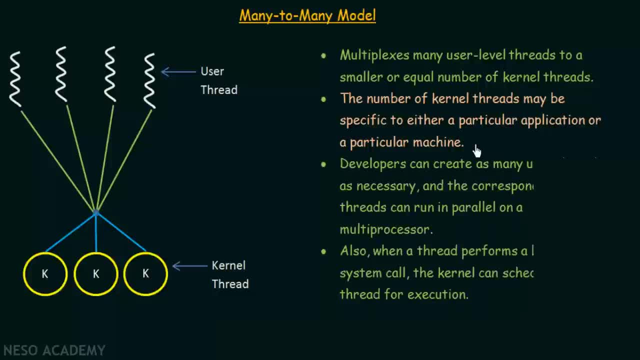 machine depending upon the number of threads that they support. And in this one, developers can create as many user threads as necessary and the corresponding kernel threads can run in parallel on a multiprocessor. So here, as we see, the developers can create as many number of. 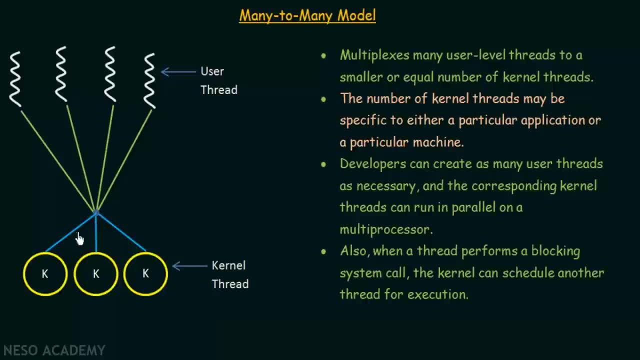 user threads as they want and they will be mapped to the corresponding number of kernel threads and they can run in parallel on a multiprocessor. So we have talked about how threads function in a multiprocessor system. So we can clearly see that in. 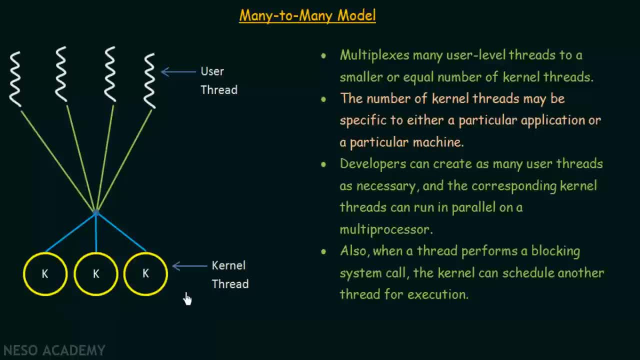 this. they can run on a multiprocessor system because we are having multiple kernel threads And also when a thread performs a blocking system call, the kernel can schedule another thread for execution. Here we see that when a user thread performs a blocking system, call the entire. 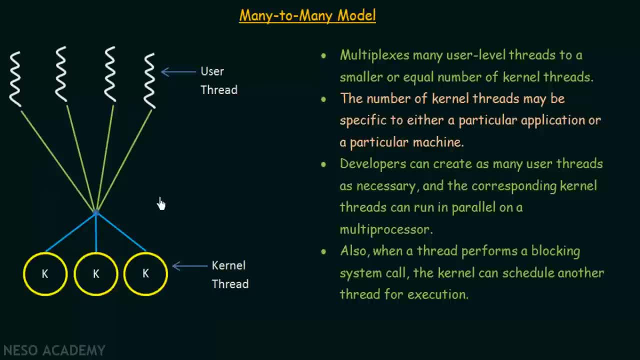 process will not be blocked. The remaining things can be scheduled for execution when one user thread performs a blocking system call. So these were the limitations that we had in the many to one model and one to one model. So in many to one model we saw 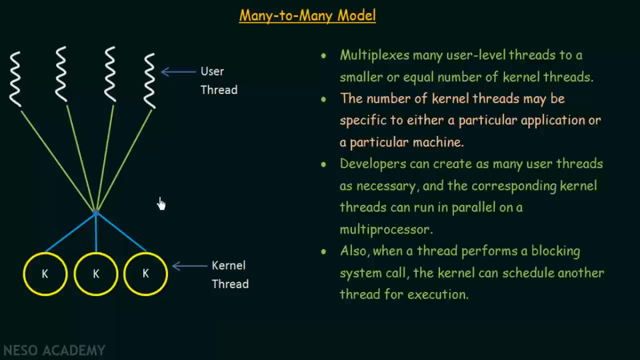 that when a blocking system call is performed, the entire process was blocked. But that problem is solved in many to many model. It was also solved in the one to one model, But in one to one model there were other problems that we faced. Like each user thread could be associated, 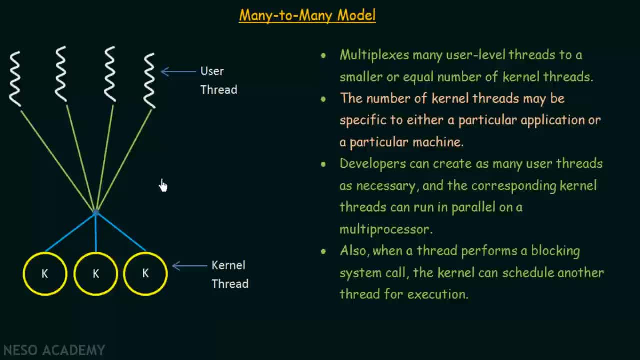 or mapped to only one kernel thread, But in this one there is a many to many relationship. So in that way also many to many model is better than the one to one model. So we see that this many to many model it is having many advantages. 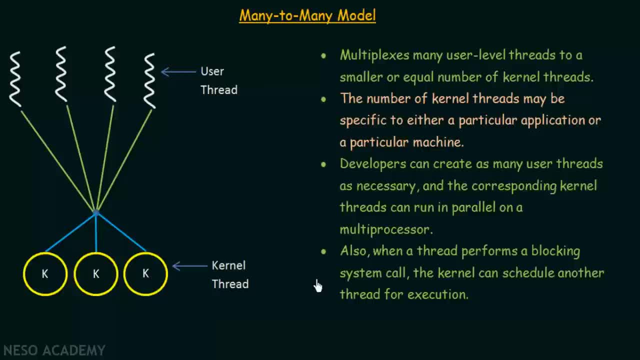 and it is far better than the many to one model and one to one model. So this is the model that is implemented in most of the systems and this is the best model that we can have in a multi-threading system to establish the relationship between: 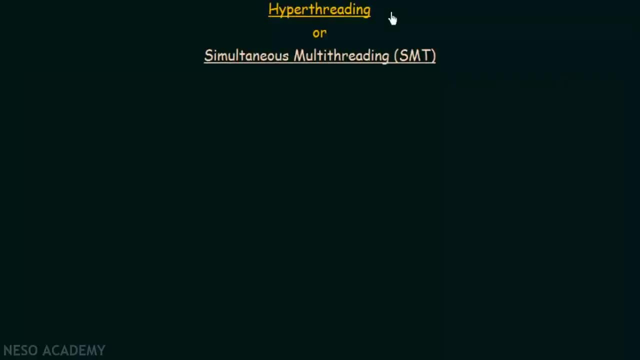 the user thread and the kernel thread. Now we will discuss another topic. that is hyper-threading, which is also known as simultaneous multi-threading. So we have been studying about multi-threading and we saw how multi-threading is much better than a single. 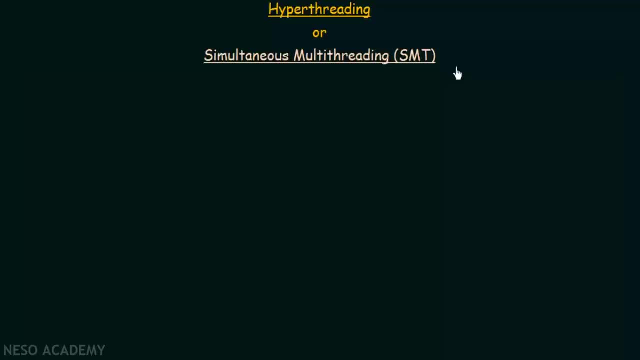 threaded process. We saw its benefits and we also saw the models in which the relationship between user threads and kernel threads are established in a multi-threading system. So what we mean by simultaneous multi-threading is that we are having more than one multi-threading. 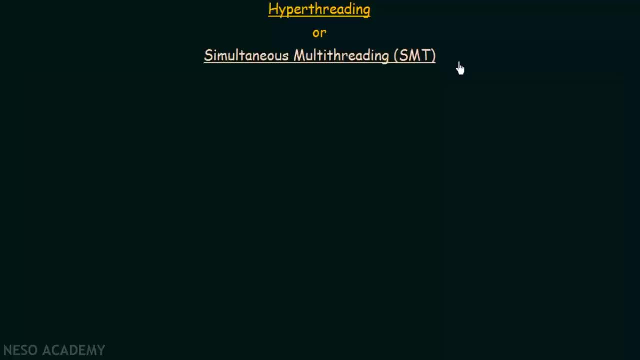 going on in the same system. Multi-threading means multiple threads at the same time, and simultaneous multi-threading means many of these multi-threadings going on at the same time. So that is what simultaneous multi-threading is And hyper-threading is the same thing. 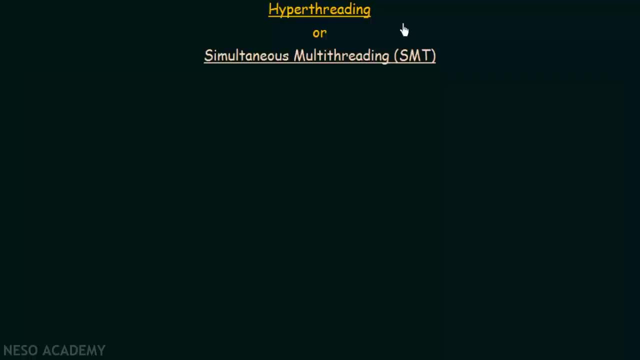 It is just the proprietary name given by Intel, So Intel company. they call it hyper-threading. So let us see what is the advantage of hyper-threading or simultaneous multi-threading, and how it actually works. What happens is that in a hyper-threaded system, 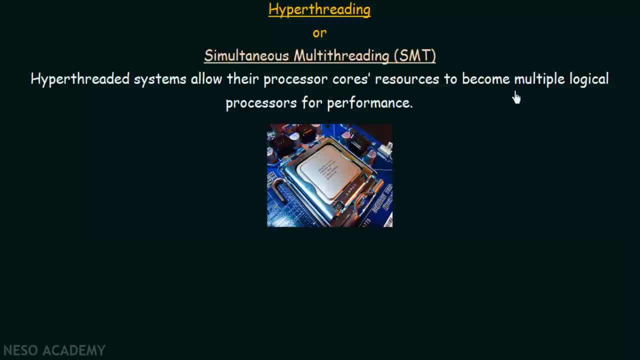 it allows their processors- cores resources- to become multiple logical processors for performance. So what we have is we are having a microprocessor. That means we are having a processor in our system where all the processing is happening, And in our processors we are having different cores. 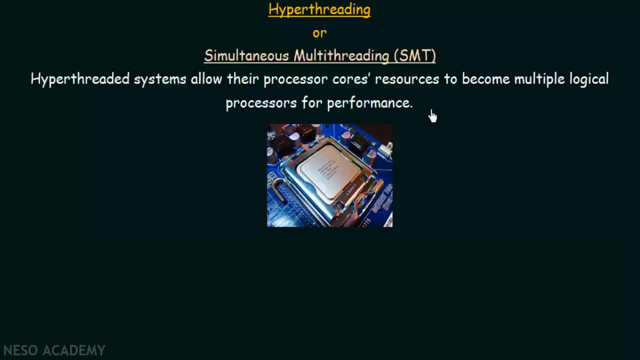 We have heard of single core systems, dual core systems, quad core systems and so on. What happens is, if it is a single core system, that means there is only one processor where only one processing can take place at a time. That means only one thread can run at a time. 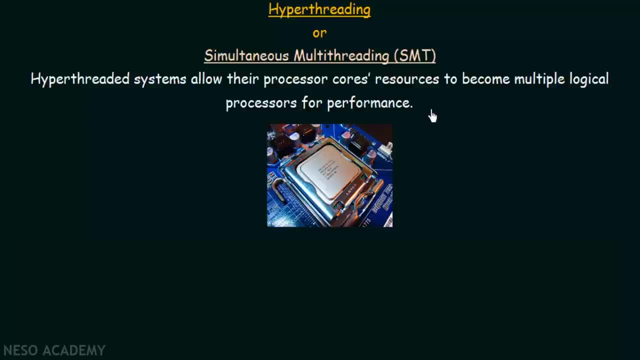 And if we are having a dual core processor, that means in your processor you are having two cores where two processings can happen at the same time. That means it will support two threads at the same time. So in the same way, quad core means four cores. 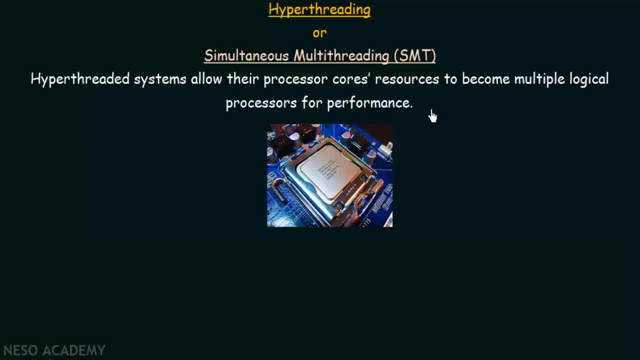 So four units of processing, That means four threads can be supported at the same time. So physically, depending upon the number of cores, you have that many number of threads it will support at one time. So in this hyper-threading, or simultaneous. 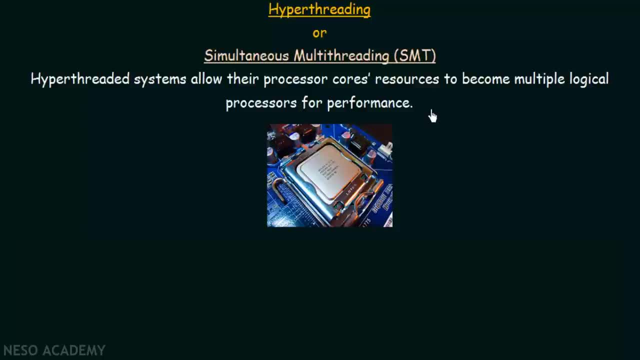 multi-threading. what happens is that the physical cores of your processors, they are virtually or logically divided into multiple processors. So if you are having one core, it may be logically divided into two. Physically it is only one, But logically it may be divided. 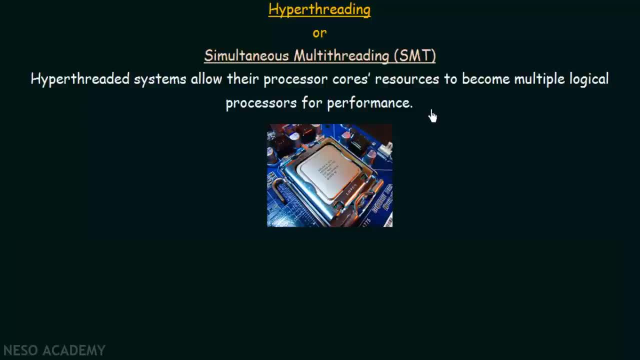 into two, So that two threads may be supported at the same time. Similarly, if you are having a dual core system, then those two cores may be logically divided into two each. So you will have a total of four cores where four different threads. 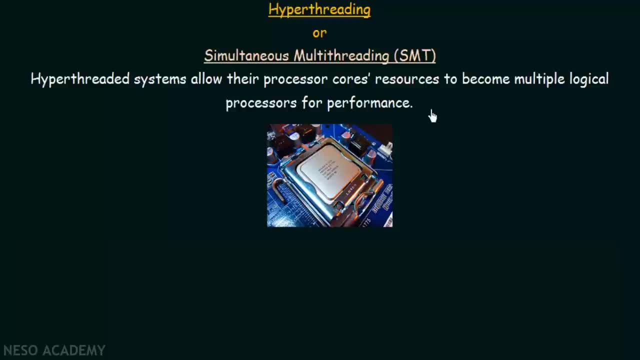 can run at the same time. So that is what we mean by simultaneous multi-threading or hyper-threading. So what happens? It enables the processors to execute two threads or a set of instructions at the same time. Since hyper-threading allows, 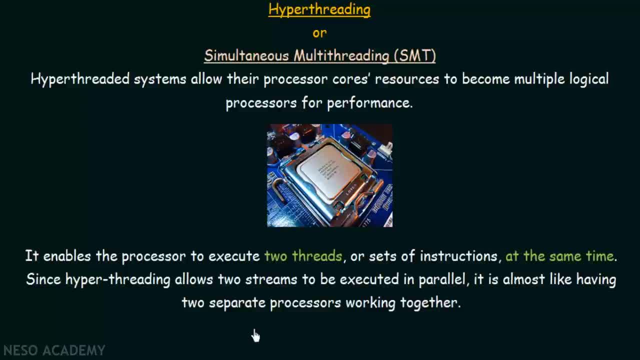 two streams to be executed in parallel. it is almost like having two separate processors working together. So this is what I just explained to you. Now let us see how can we find out if your system that you are using supports simultaneous multi-threading or hyper-threading. 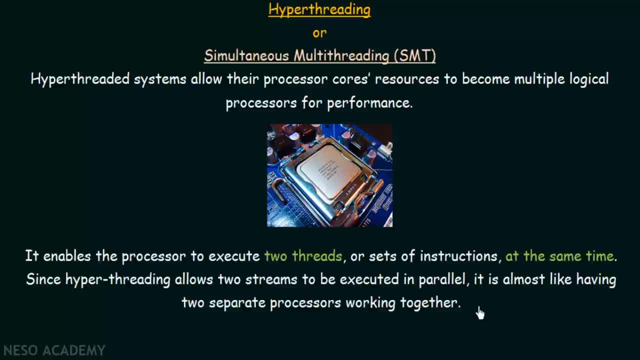 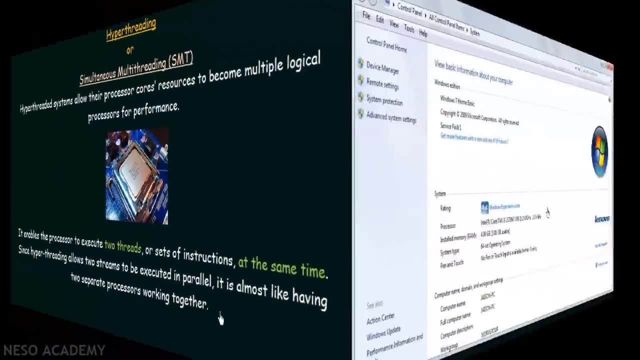 And let us see how we can find out if hyper-threading is running in our system, Because it is always interesting to practically see what is happening instead of just learning the theory. So let us try to find out how this works. So here I just want to show you. 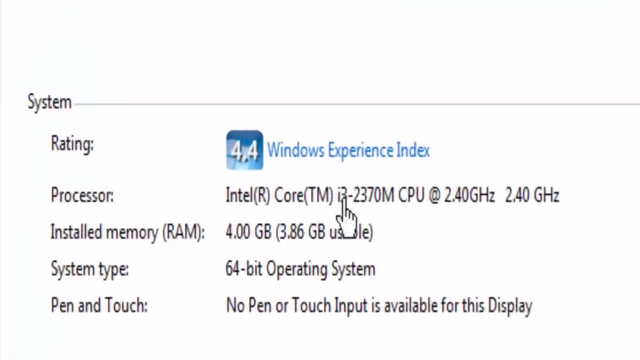 the properties of the system that I am using right now. So here I am having a processor which is of Intel Core i3 and it belongs to the 2370M model. So this is the processor that I am having in my system right now. 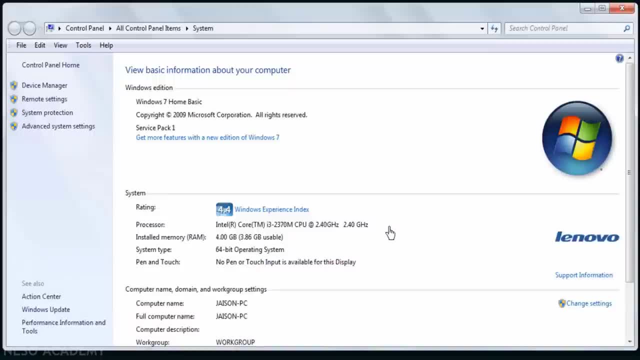 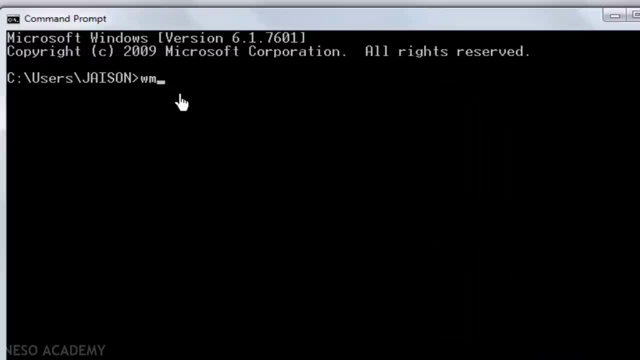 So, in order to find out whether my system is hyper-threaded or not, what you have to do is you have to open your command prompt. So you open up your command prompt and here you type WMIC. So WMIC stands for. 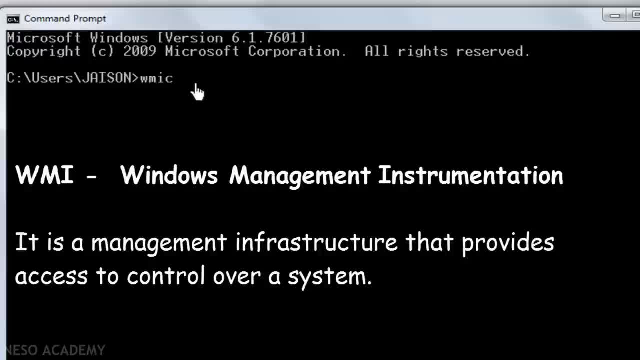 Windows Management Instrumentation, which is a management infrastructure that provides you access to control over a system. So if you type WMIC, it will open up the Windows Management Instrumentation console. So if you press enter you enter the command line interface of WMI. 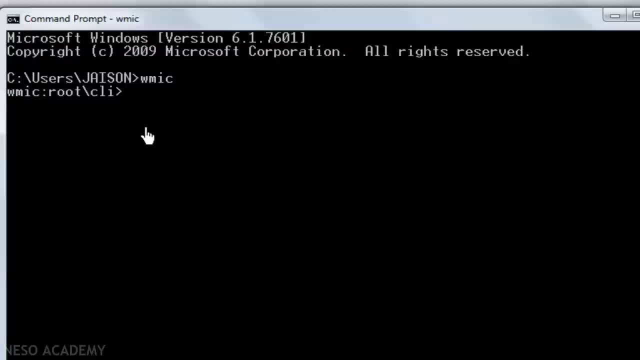 So here I will show you the command which will help us know how many cores are we having in our system. So here there is a command called CPU, get number of cores. If you type this command, it will show you the number of cores. 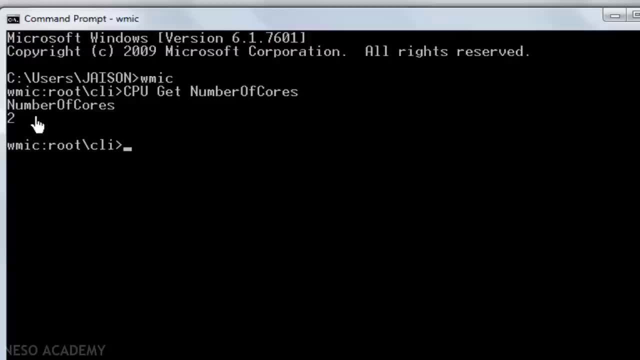 that you have in your system. That means the number of cores in your processor. So we know there are different types of processors having different cores And, as I told you, I am having two cores in my system. So here you see that. 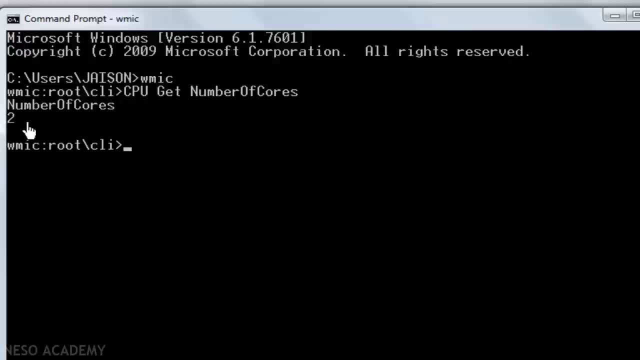 I am having two cores in my system. That means there are two threads that can be supported at the same time, So it is just like having two processors. Now we will find out how many logical processors do I have Now. if the number of logical processors 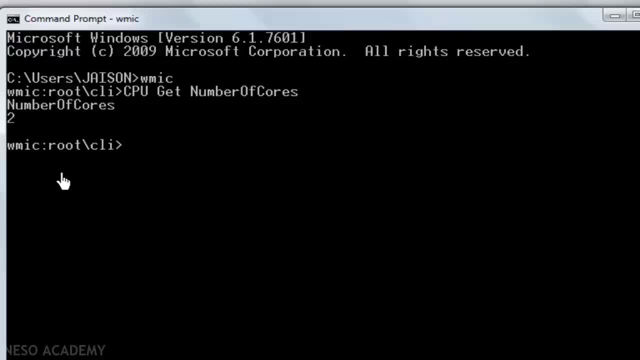 is equal to the number of physical cores. that means there is no hyper threading happening in my system Because I am just having that many number of cores as the physical cores that I have. But if I am having more number of logical cores compared to the physical cores that we saw here, 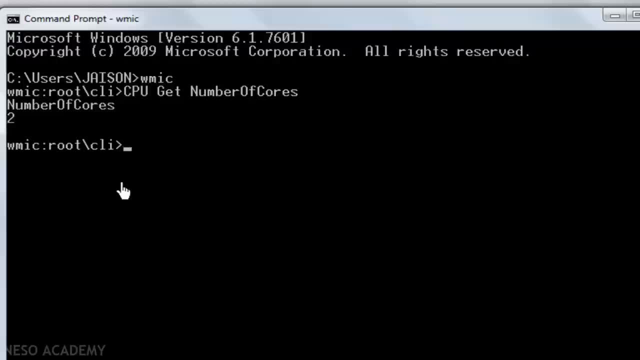 then that means hyper threading is happening in our system. So in order to do that, there is another command. So let us extend this command. Here we said: get number of cores. Now we will also say number of logical processors.